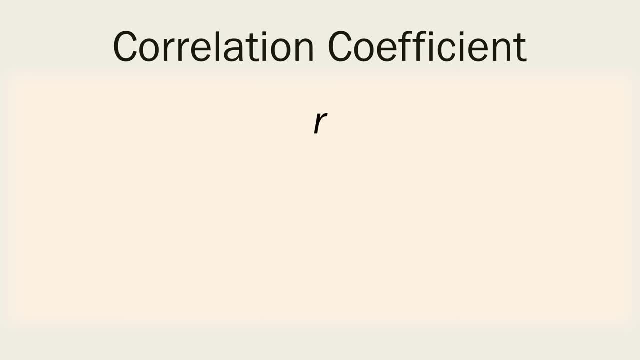 r. It is represented by the letter r. It can take on values only between x and y. It is between negative 1 and 1. And it describes both the strength and the direction of the relationship. The absolute value of r tells us about how strong the relationship is. 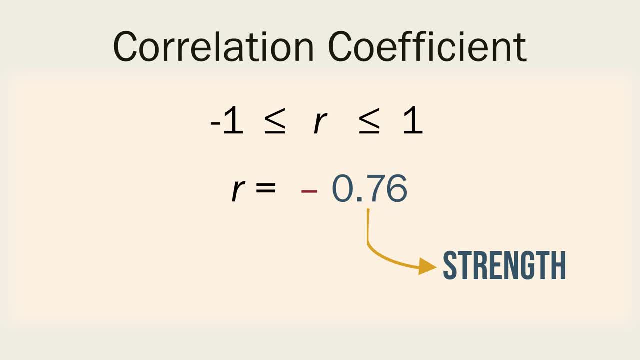 The stronger the correlation, the larger the absolute value of the correlation coefficient. The sign on the coefficient, positive or negative, tells us about the direction of the relationship. So when r is negative, 1. We have a perfect negative correlation. And when r is positive, 1. 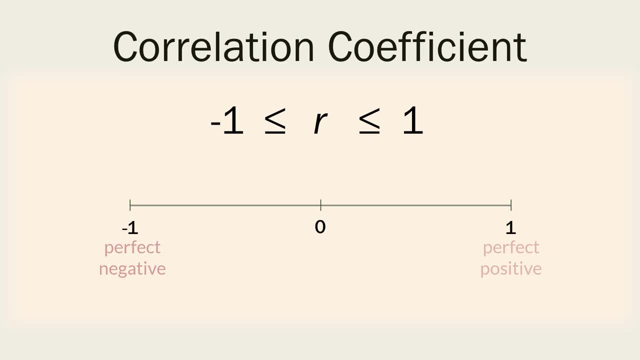 The relationship is positive and perfect. The closer r is to negative- 1 or 1,- the stronger the correlation. The closer r is to 0, the weaker the correlation. And when r equals 0, we say there is no correlation. 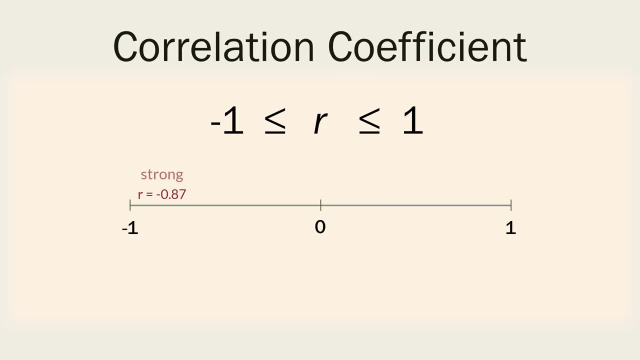 So r equals negative .87 will be considered strong. r equals 0.42.. We have a perfect negative correlation: r equals 0.13 will be moderate and r equals 0.13 will be considered weak. There is no general agreement on what values of r represent: weak, moderate and strong correlation. 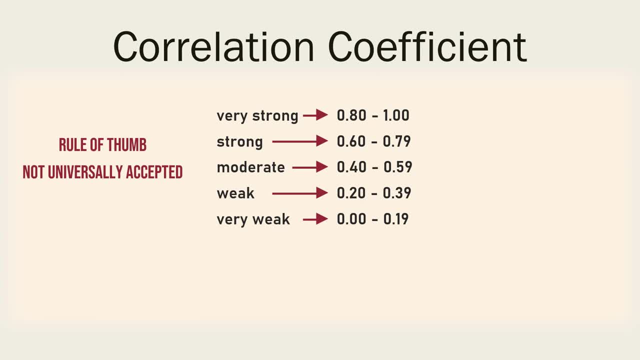 because of several other factors, like sample size. In some cases r equals 0.5 is considered moderate, While in some cases it is considered strong. So I will leave it to you to check your textbook or course for their guideline on how to categorize. 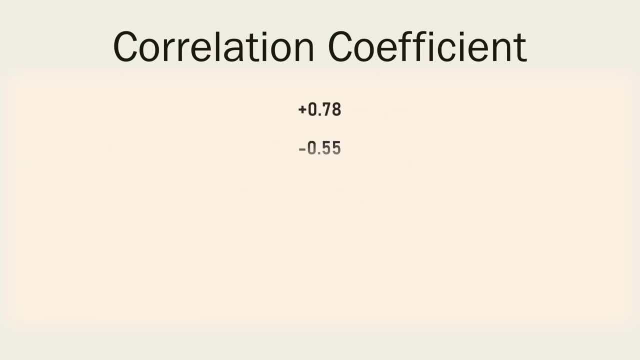 correlation strength. Now let's look at a quick question: Which of these correlation coefficients indicates the strongest correlation? The highest value here is positive, 1.23, which unfortunately cannot be a correlation coefficient because it is greater than 1.. So the answer is negative, .87, because it has the largest absolute value between negative. 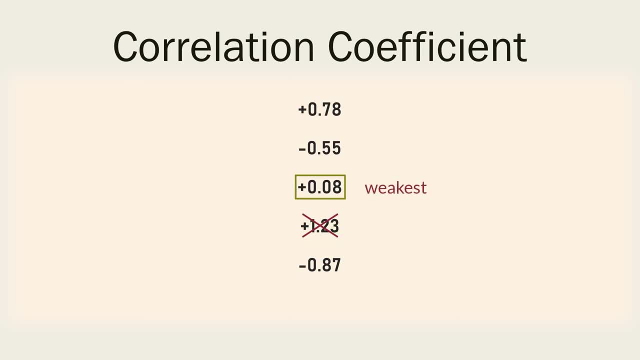 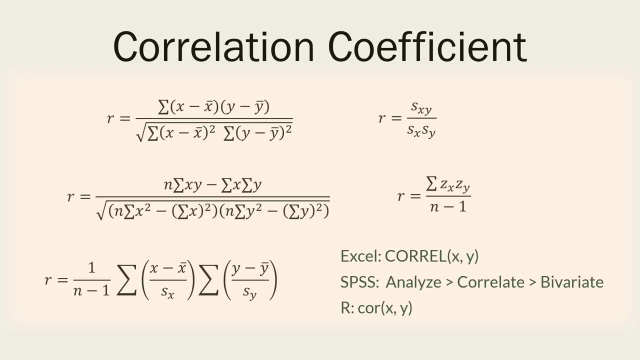 1 and 1.. And the weakest will be positive 1.23.. So the answer is negative .87, because it has the largest absolute value between negative 1 and 1.. The correlation coefficient can be calculated in different ways depending on what is available. 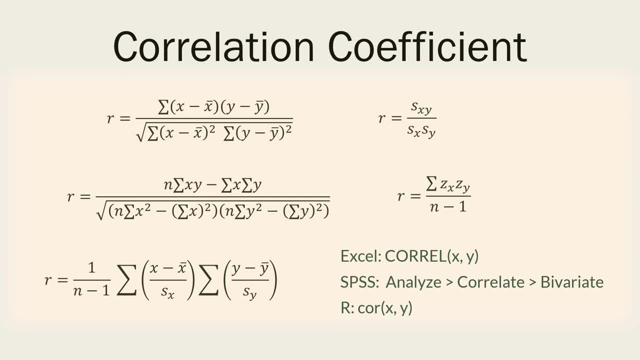 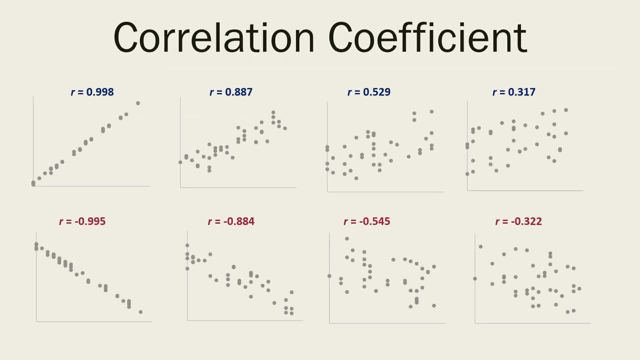 either by using formula or software. Note that swapping the positions of x and y here does not change the value of the correlation coefficient. That is, the correlation between x and y is the same between y and x. Here are some scatter diagrams with their corresponding correlation coefficients. 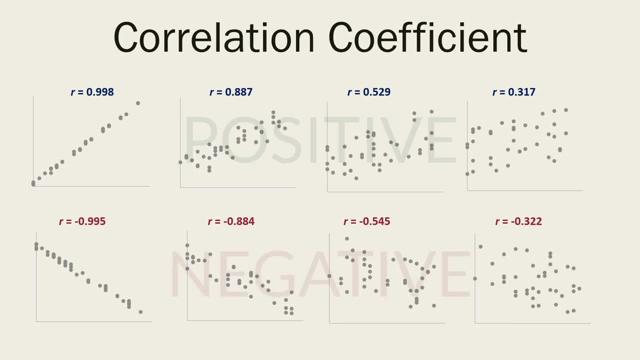 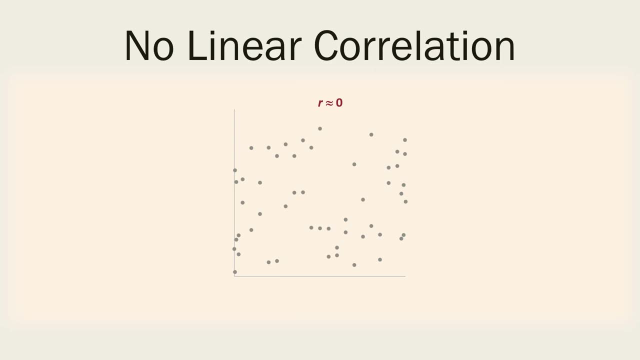 Positive correlations at the top And negative correlations at the bottom, And here we have practically no correlation, as it is difficult to approximate these points by a single straight line. These curves and circle, however, show some clear relationships, But none of them can be well represented by a straight line. 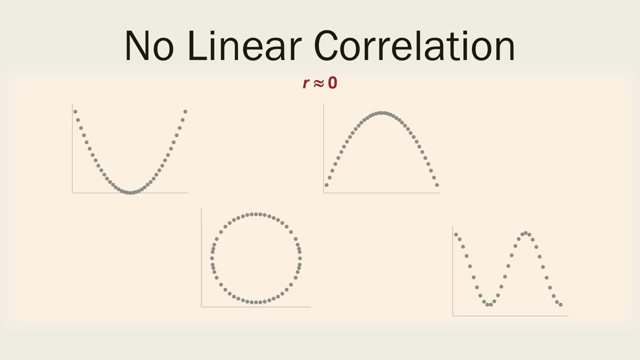 So as far as correlation is concerned, here, the correlation coefficients for these are approximately zero. Now consider this case where the points Clustered together enough to be represented by a straight line, Would you expect the correlation coefficient to be close to zero, or to one? 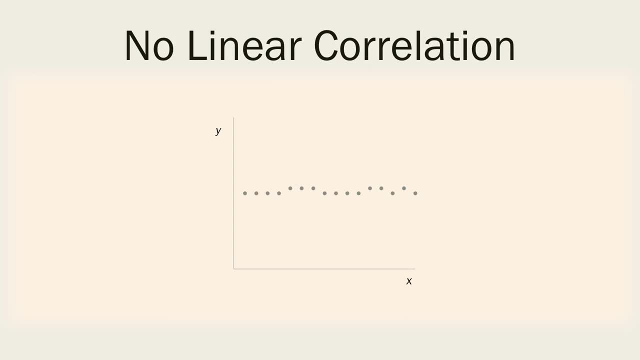 You might say one, because the graph satisfies the straight line requirement, But that would be incorrect because the values of y are neither increasing nor decreasing as x increases, That is, the values of y are pretty much constant, So the correlation would be close to zero. 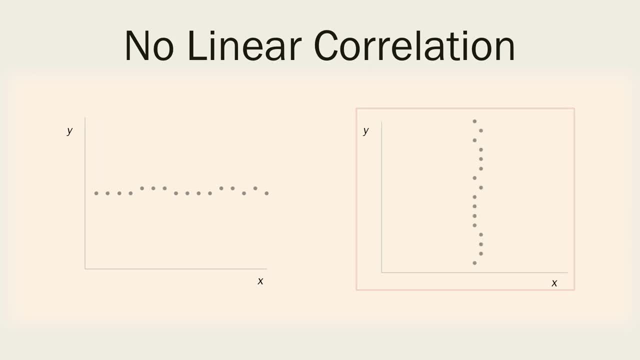 Likewise here The correlation is close to zero because y increases and decreases without x changing in value. Now if two variables have a strong correlation, we do not say that one affects or causes the other to change without further analysis. For example, if there is a strong positive correlation between class attendance and grades. 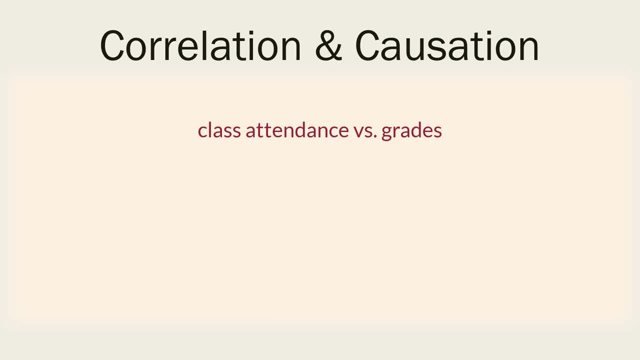 we do not conclude that class attendance causes grades to increase. It is possible that the same students who regularly attend classes will have a positive correlation, But if the same students who regularly attend classes also consistently do their own work, watch related videos and do a lot of practice, 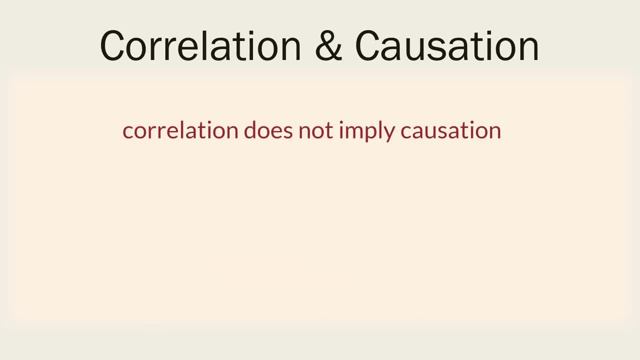 So correlation does not imply causation or causality. We can say that as class attendance increases, grades also increase, But we do not say that increase in class attendance causes grades to increase. That is without performing an experiment. So to wrap it up, 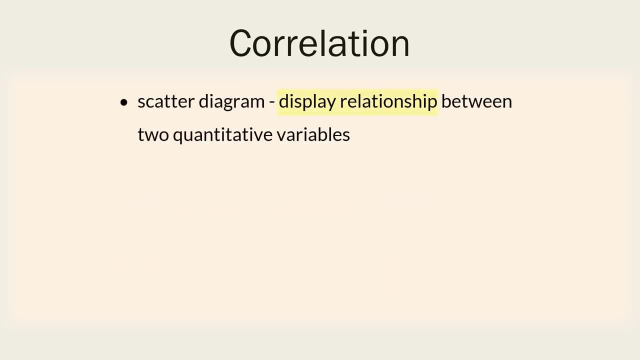 We looked at how scatterplot works. Scatterplots are used to display relationship between two quantitative variables. We showed that correlation coefficient r is a number between negative 1 and 1 and is used to describe the strength and direction of a linear relationship. We stated that correlation coefficient can be obtained using formula or software, and.